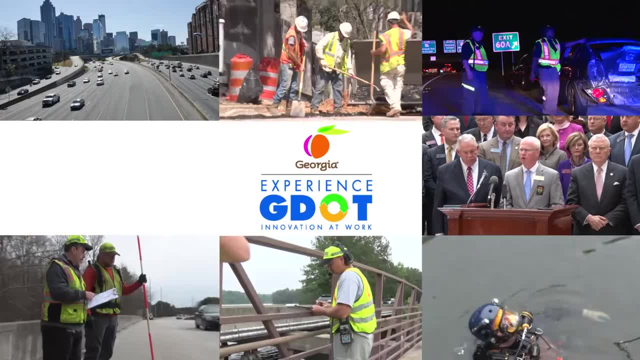 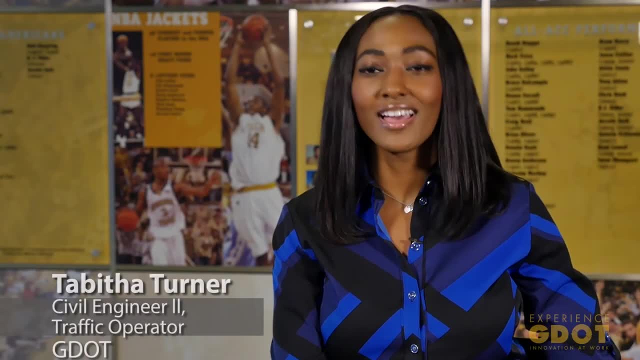 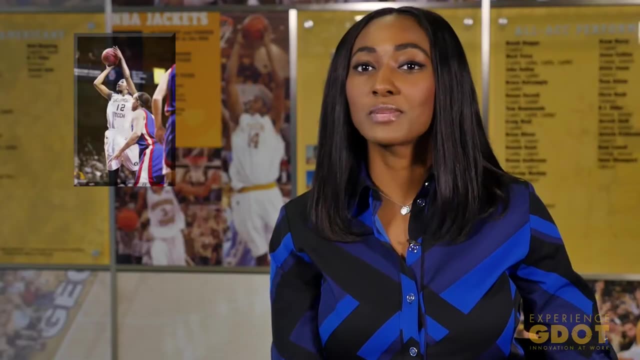 Hi, my name is Tabitha Turner. I'm a level 2 engineer for the Georgia Department of Transportation. I graduated from the Georgia Institute of Technology with a bachelor's in civil engineering and business management. There I played women's basketball for four years and I also pledged. 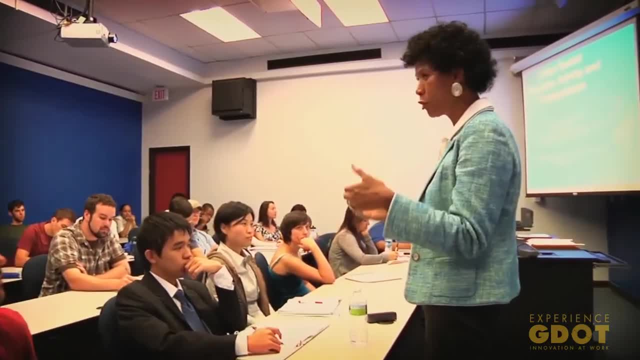 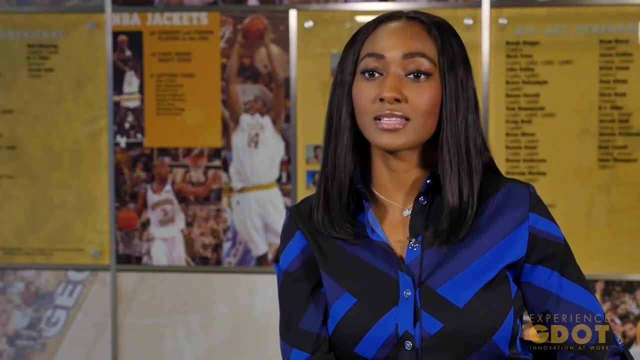 Alpha, Kappa, Alpha, Sorority Incorporated. Some of the classes that help with the transportation engineering career that I'm in right now are definitely going to be a lot of your transportation classes like design and community planning, roadway design. You've got a lot. 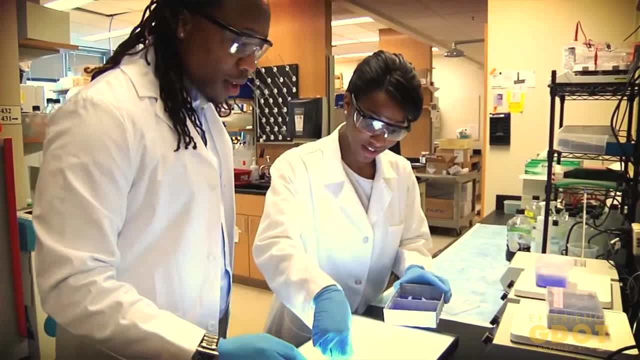 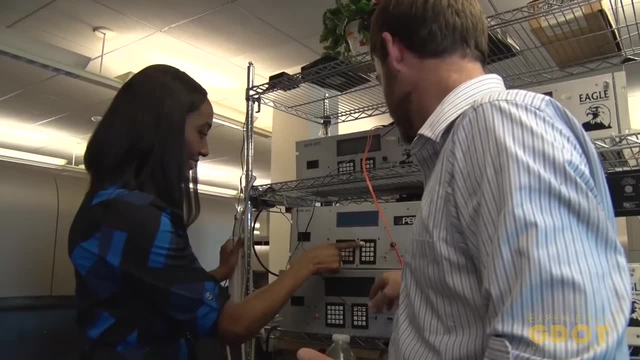 of structural classes, fluids, classes that help with waterways, and engineering. You need all that to be a transportation engineer. My day-to-day consists of taking old systems and trying to update them and make them new, because some of the old GDOT systems were. 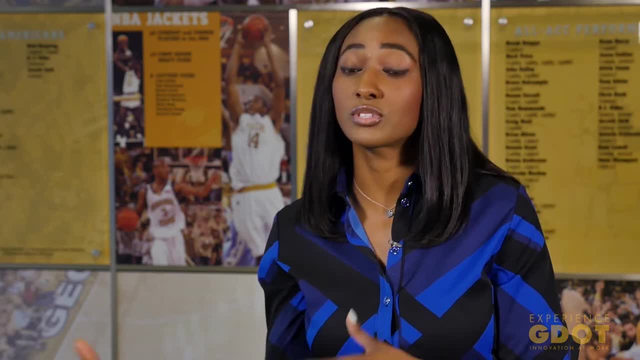 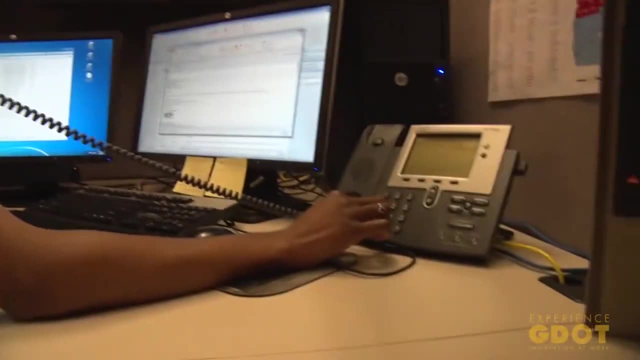 a little archaic and we're trying to bring them back into the millennial generation. I do everything from cost estimates on a daily basis, where we, from the beginning, we're trying to find out how much money each project takes to build, and we go back to our supervisors. 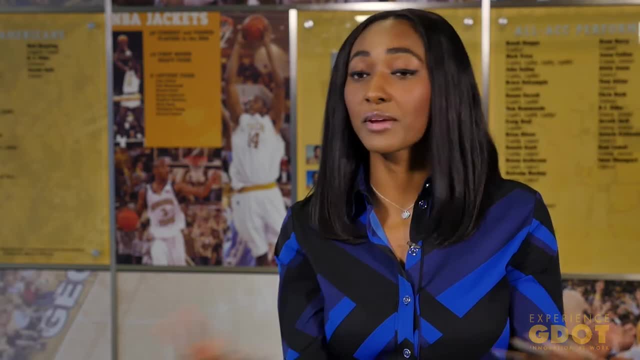 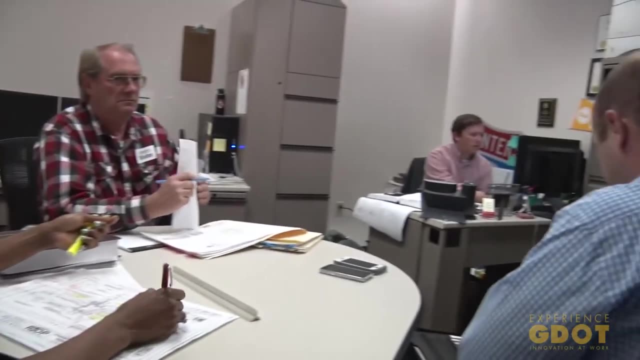 and get the funding for it. I also do micro station and auto cad work where if there's something wrong in the plans that doesn't correlate in the field, we have to update those and put them in. So the best thing about my job I can honestly say is being able. 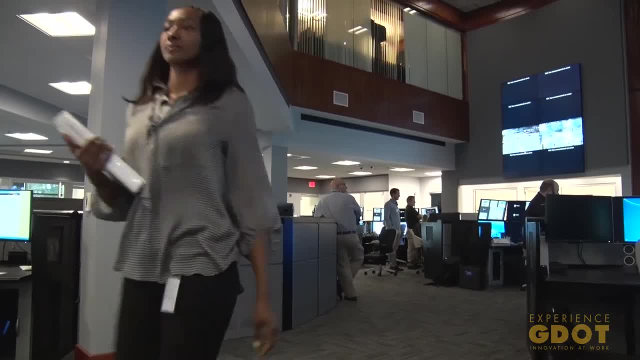 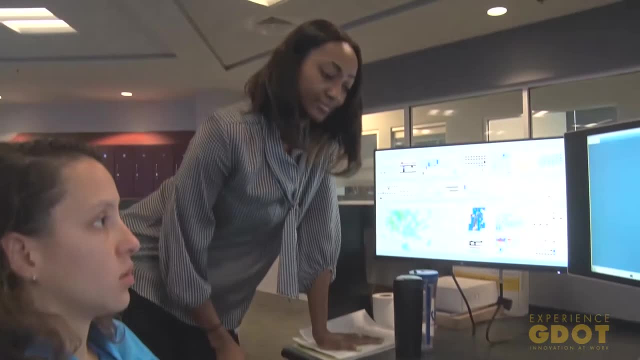 to directly see the benefit that I provide to the public, And I know that sounds a little cliche, but it's one of those things where, okay, if there's traffic at a signal and we call in and they say, okay, I'm backed up at this light for about an hour or two and 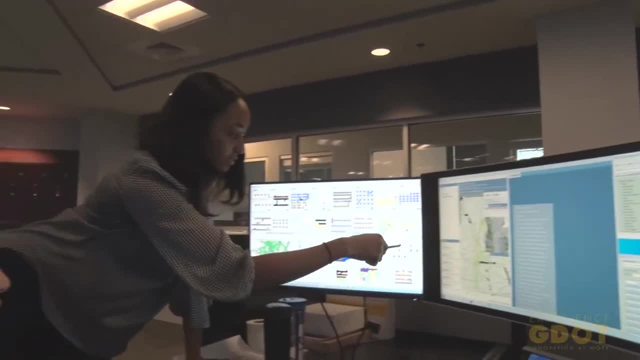 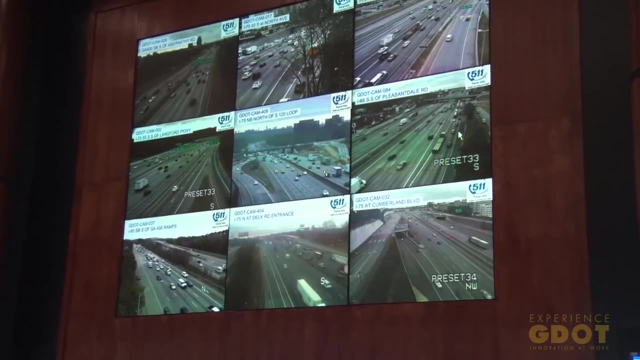 I can't get through. they call in and we go and we look at the system and we can reprogram and re-time the lights and they see a direct benefit right there And you know it might be something that's really minuscule, but when you're the person that's sitting there in 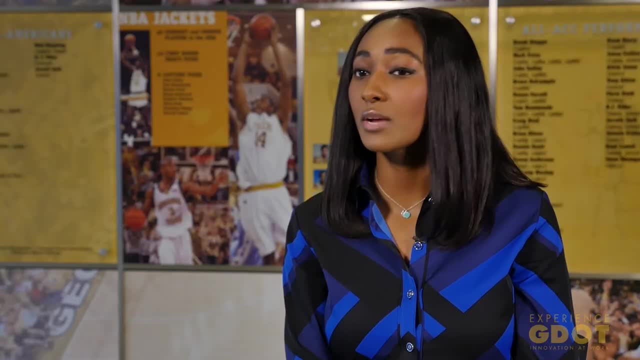 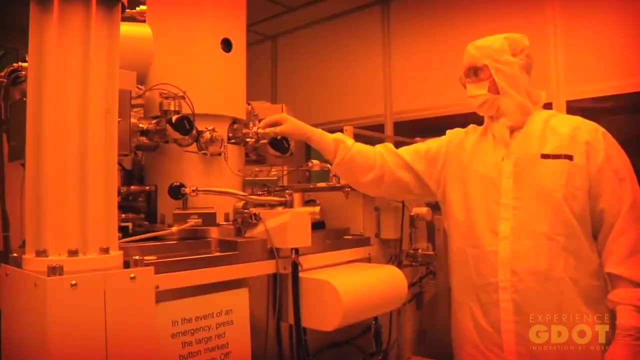 traffic. it makes a big deal to you, right. Another piece of advice that I would give myself would be to intern or co-op while you're in school, because when you get out you can have a job waiting for you. Oh, and also take your EIT. 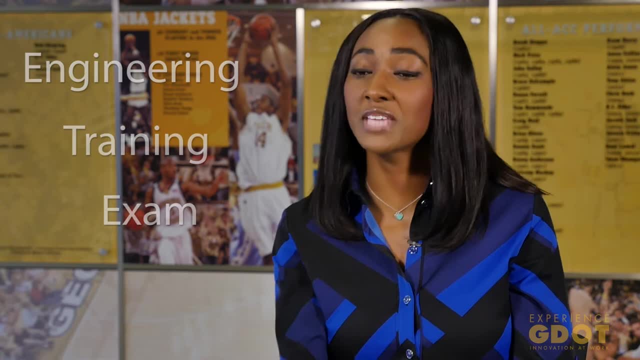 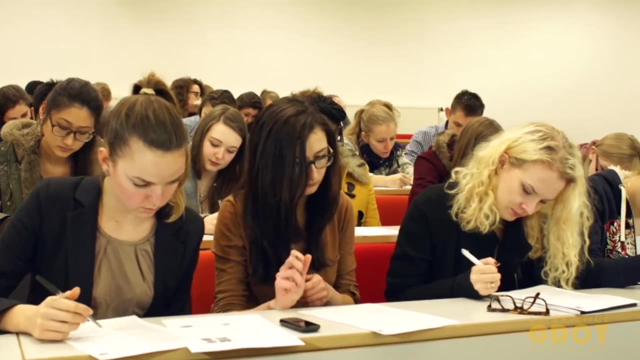 Which is the engineering training exam. And when you do take it before you get out of school, take it seriously, because taking it- or should I say waiting to take it after you graduate becomes hard, because you start to forget everything that you learned while you.